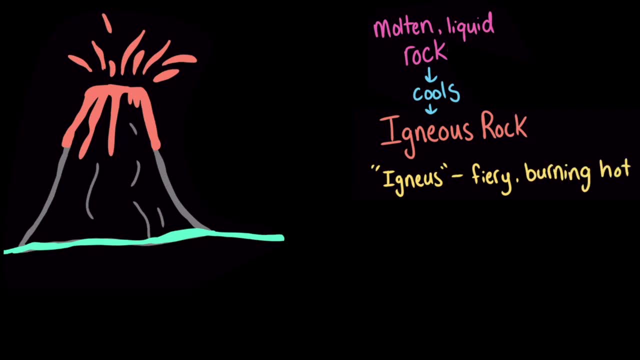 Igneous rock is a rock made of molten rock. Igneous rock is a rock made of molten rock. Igneous rocks make up more than 90% of the earth's crust. One common kind of igneous rock is granite, which you've probably seen in bridges. 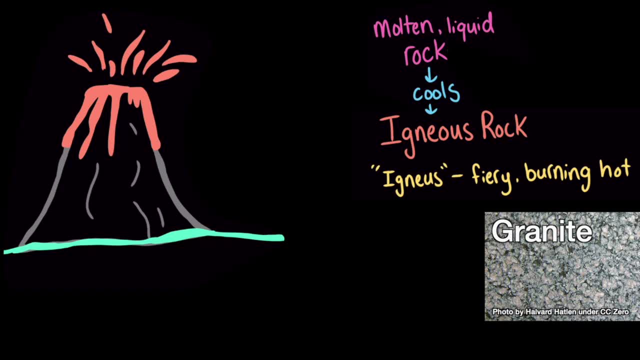 buildings and countertops. Another kind of igneous rock is obsidian, which is smooth and glassy and is sometimes used to make knife blades. Both of these rocks were made of molten rock, So why do they look so different? Well, granite was made from magma. 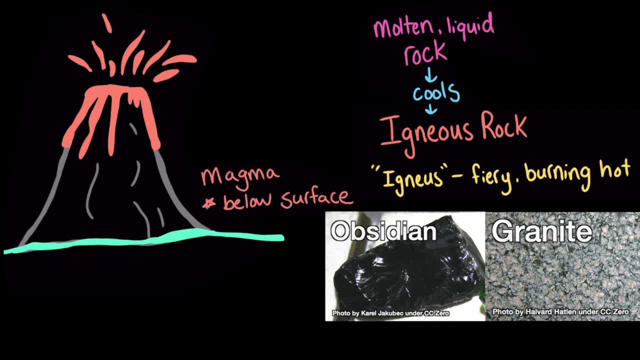 which is molten rock that exists below the surface of the earth. Magma tends to cool slowly underground, which gives time for the elements in it to form large crystals, And this obsidian rock was made from lava, which is molten rock that flows above the ground. 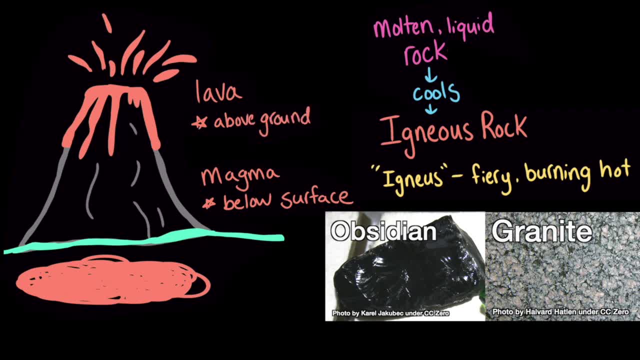 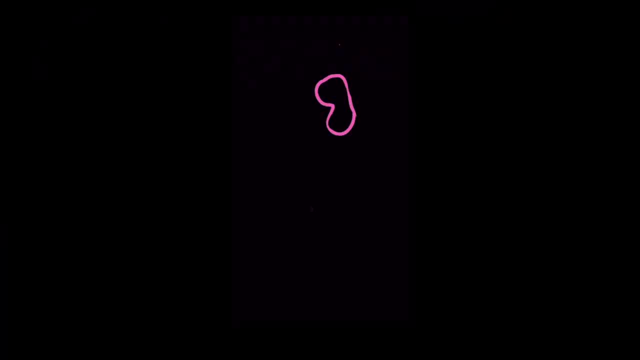 Lava tends to cool quickly, which causes the rocks it forms like obsidian to have smaller crystals. I always remember the difference between magma and lava. like this, I keep my lava lamp above the ground, just like lava is above the ground. 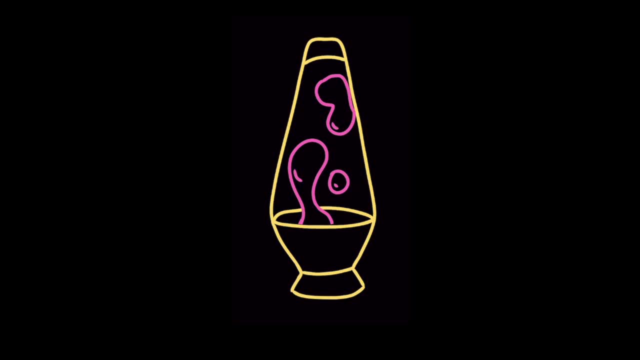 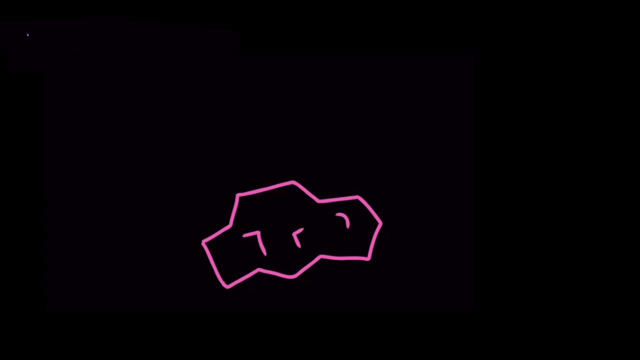 If I buried my lava lamp in the ground, then I can call it a magma lamp. Once an igneous rock is created, its journey isn't over. The rock might begin to change through a process called weathering. This is when water, weather, wind and other physical forces chip away at a rock. 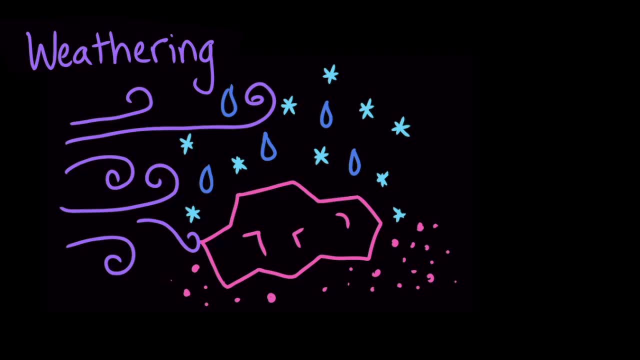 and cause little pieces to break off. These little particles are called sediments. The sediment from our igneous rock can be moved around by wind and water. This is called erosion. Eventually the sediment will settle down somewhere, maybe at the bottom of an ocean or a lake, And it might join other sediment from other rocks. 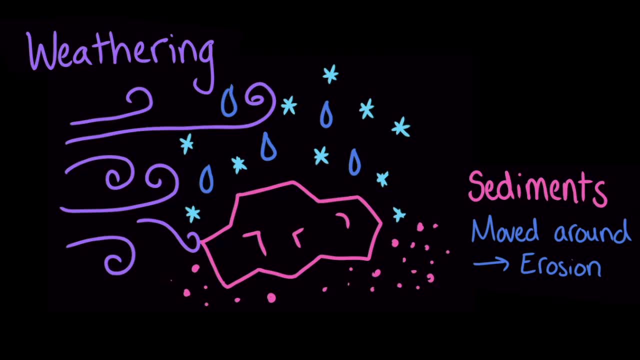 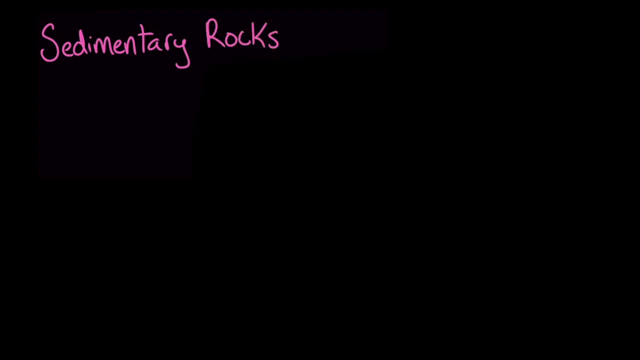 crushed up shells and plant matter And over time this sediment will become a rock. Rocks that are formed from sediments are called- you guessed it- sedimentary rocks. But how does sedimentary goop at the bottom of a lake become a rock? 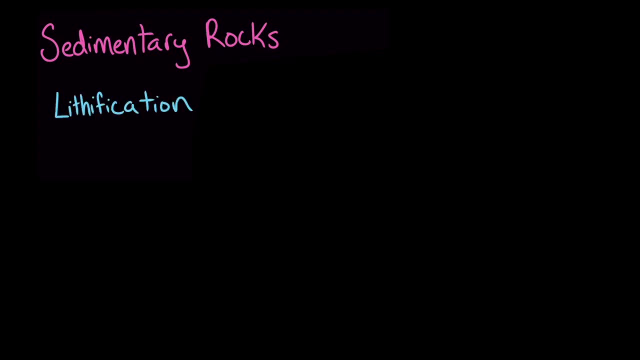 Well, it goes through a process called lithification. Lith comes from the Greek word for stone, So you can think of this process as stonification. The first step of lithification is called deposition. This is when sediment is deposited in a new location And it spreads. 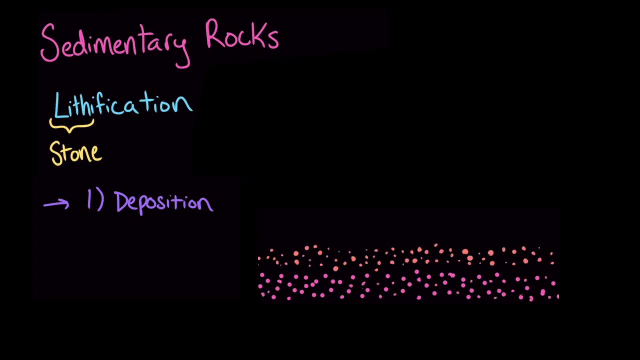 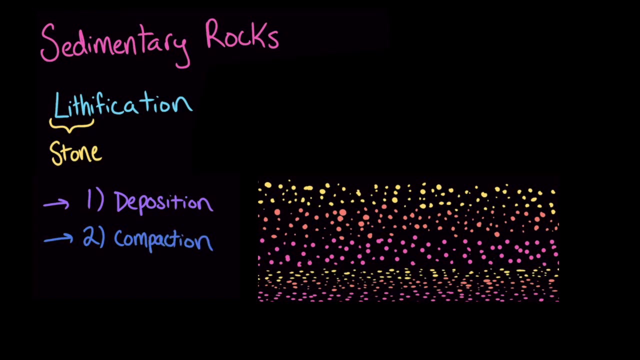 out to form a layer. As more and more layers are created, the layers underneath them become squished together. This is called compaction. When water moves through the layers of sediment, it can carry dissolved minerals with it. The water can leave these minerals. 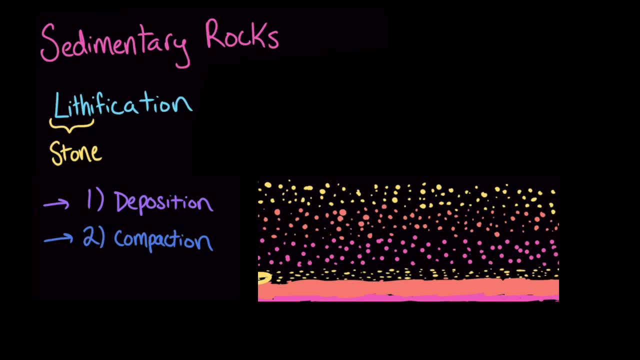 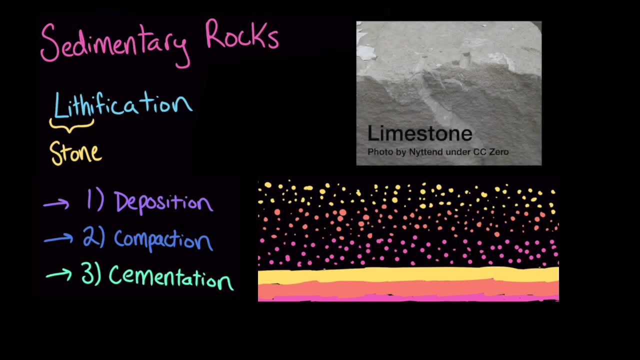 in between the sediment particles, which makes everything stick together. This cementing of sediment is called cementation. Limestone is a sedimentary rock that is made when sediment that contains a lot of calcium carbonate in it goes through lithification. But once a sedimentary rock has been created, it doesn't mean that it is done changing. 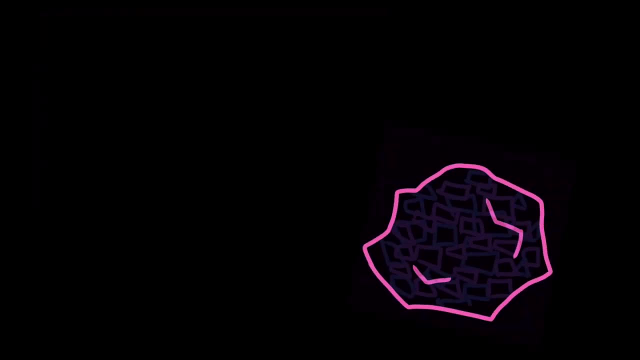 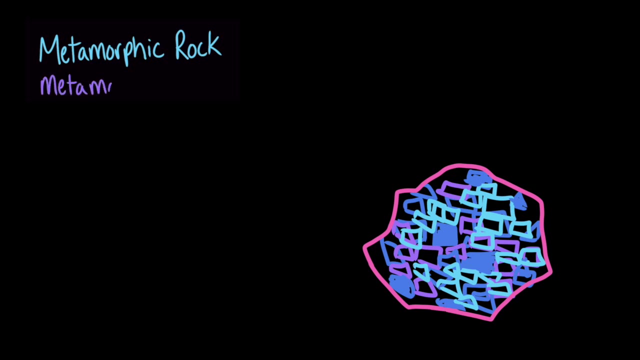 Sometimes a rock is squeezed or heated so much that the minerals inside it actually change composition. It is now a metamorphic rock. You might have heard of the word metamorphosis, which describes when something changes from one form and structure to another, Like when a caterpillar turns into a butterfly. Metamorphic rocks are made when igneous. 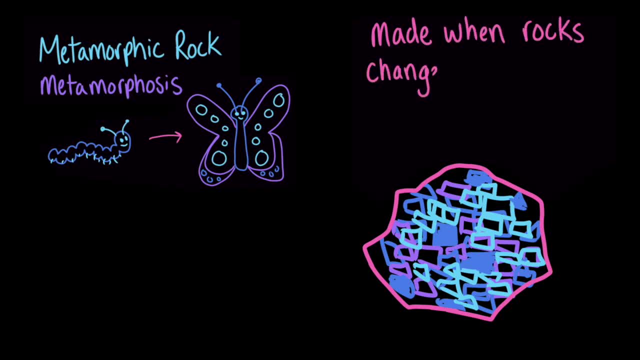 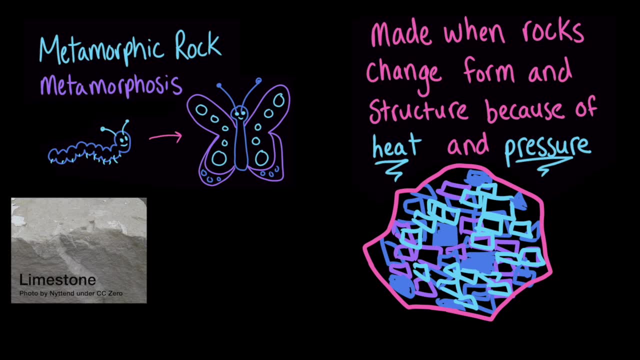 sedimentary or even other metamorphic rocks change form and structure Because of heat and pressure. When the sedimentary rock limestone gets put under a lot of heat and pressure, it can turn into marble, But metamorphic rocks still might not be done. changing Rocks can. 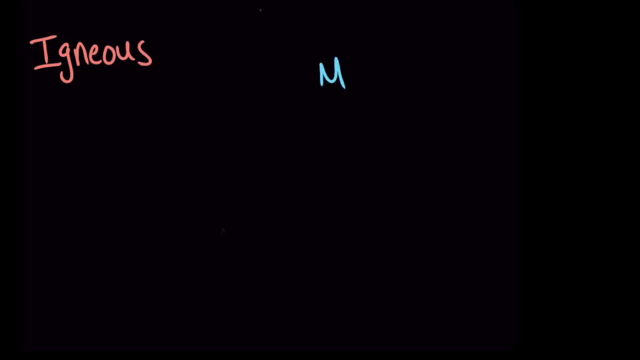 actually keep on changing forever. Igneous metamorphic rocks can actually become sedimentary rocks if they are broken apart into sediments when they go through lithification. Metamorphic rocks and sedimentary rocks can become igneous rocks when they are melted. then cools Egneous rocks and 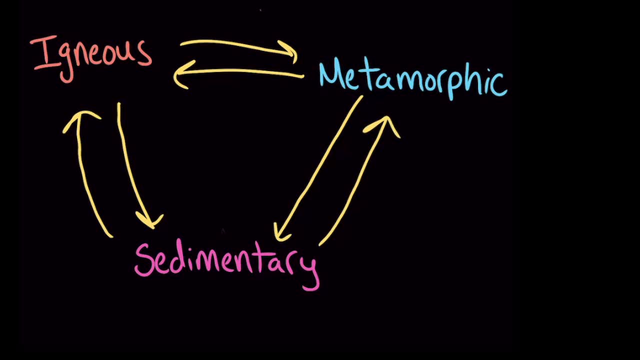 sedimentary rocks can become sedimentary rocks when they melt, then cool down. Roaches can can become metamorphic rocks when they're exposed to high heat and pressure. This is called the rock cycle, So maybe next time you get the chance to stare at a rock. 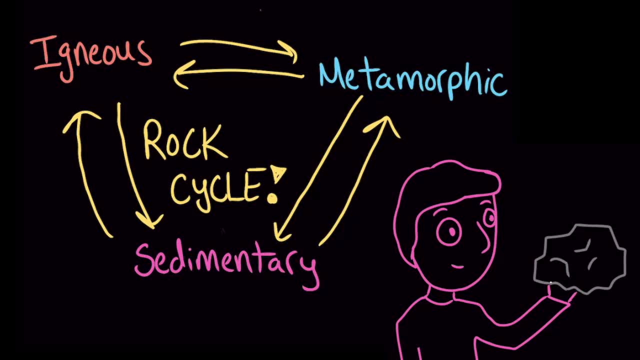 see if you can figure out whether it's igneous, metamorphic or sedimentary. And when rocks change so much, who knows what kind of rock it'll be next?